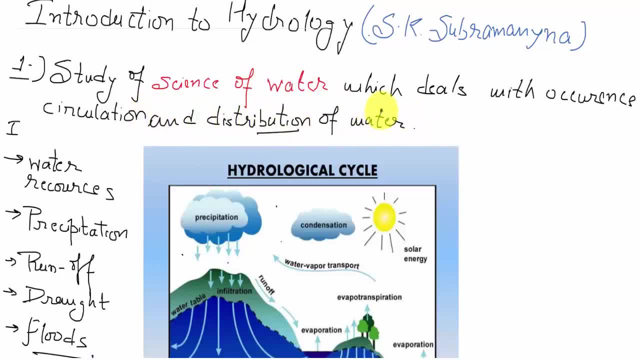 circulation and distribution of water. Occurrence means how does water on the earth and in various forms, how does it come to be, how does it occur? Circulation means how does this form of water circulate from one place to another place, and distribution means what is the ratio? 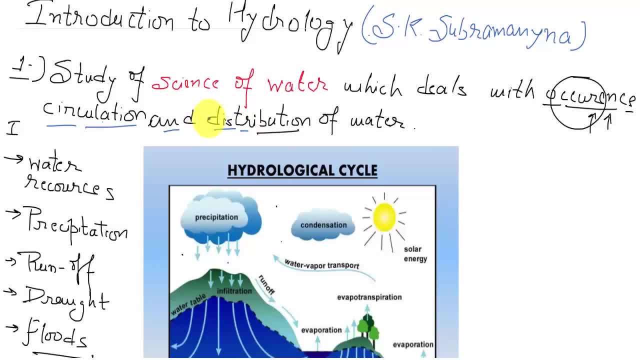 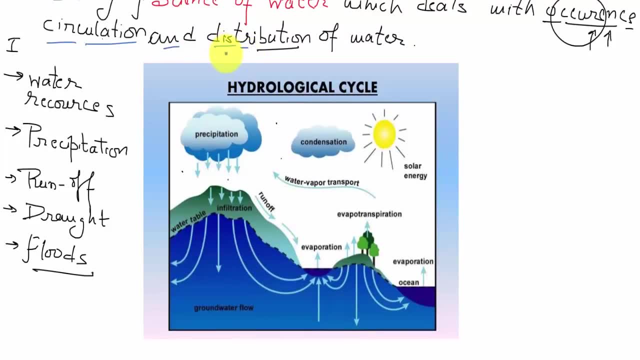 in which various components of water. what is the ratio in which various components of water are distributed? Basically, hydrology begins the study of basic cycle called as hydrological cycle, The cycle we have a prime source of energy, which is our sun. It also 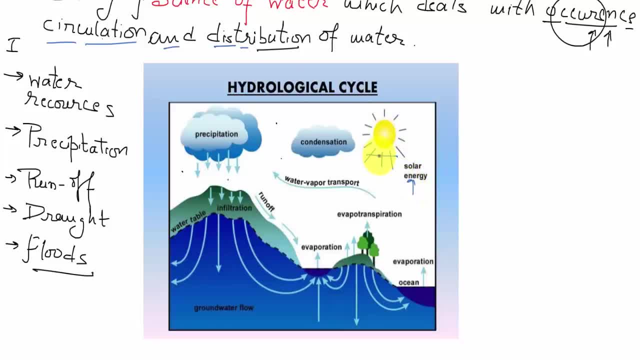 gives us solar energy, and it is through the energy of sun that we get to drive this hydrological cycle. So the cycle begins like this: We have sun, which emits radiation, and it emits the energy of the earth As soon as it reaches earth surface. there are water bodies such 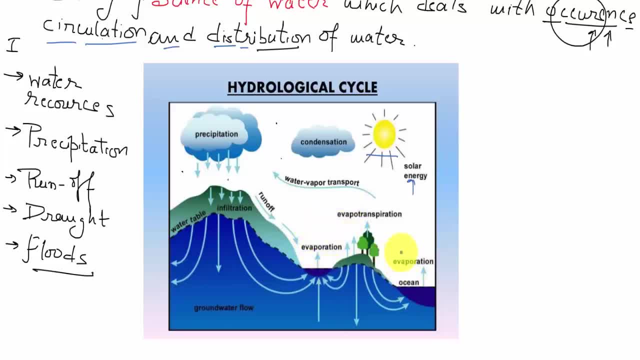 as oceans, lakes and rivers. From these water bodies we have a process called evaporation. Evaporation is the process where water molecules leave the water and enter into a vapor state. Now water vapor is transported and it becomes cloud. After the temperatures comes down, there is a process called as precipitation- Precipitation. 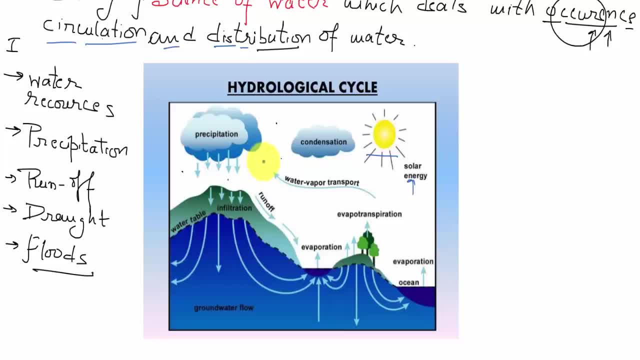 does not mean that it will only rain. Precipitation may occur in various forms, such as rain, snow, hail and other forms. So, due to the condensation of water vapor, which was earlier part of ocean, now we have water molecules from sea. 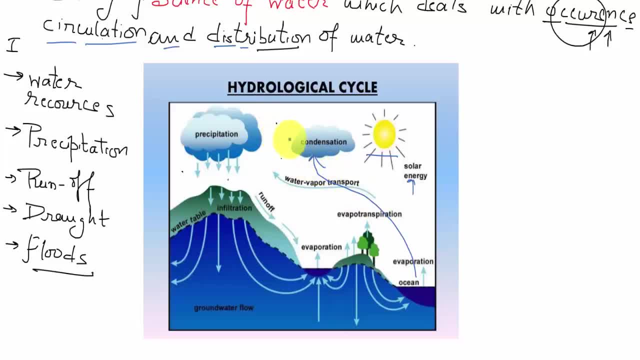 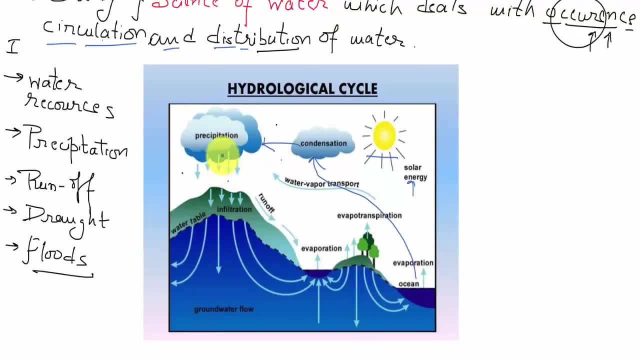 We have water molecules from sea right upto the clouds, and then from clouds we have our own precipitation cycle. So after the rain, this is our earth surface. There will be two things: a waterfall here, Then either it may run off- It means that- either it may go along. 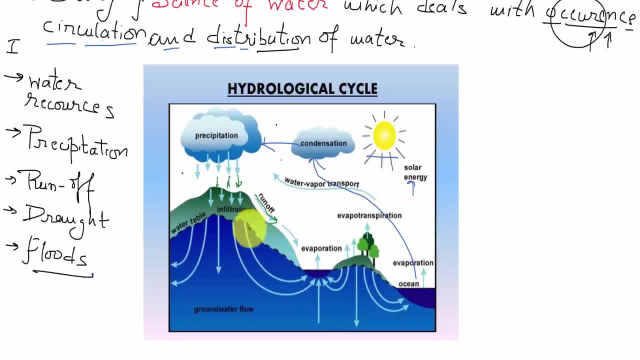 the slope or it may come down into the earth surface. So the water which goes along the earth surface is called as a runoff and water which comes into earth surface is called as infiltration. Now the runoff portion keeps on coming and somewhere it meets a water body. It may either be a lake or ocean or river. 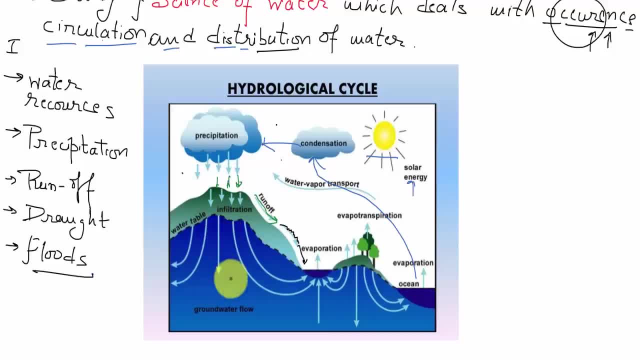 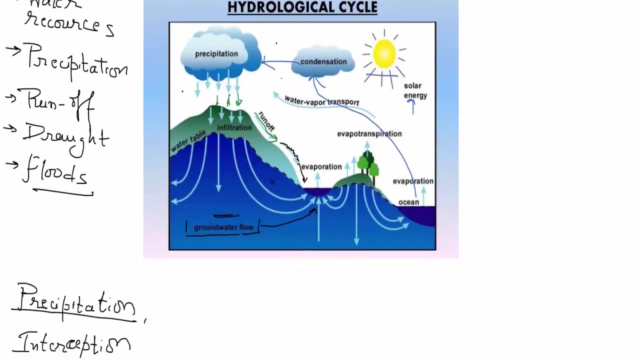 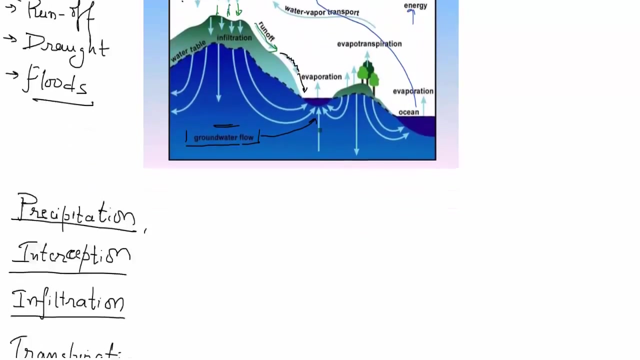 Now the part which has infiltrated it becomes a part of groundwater. Groundwater is that water which is stored in the form of water at the ground, below the ground. So this groundwater also contributes to water bodies such as river. We will look at various terms in this hydrological cycle so that meaning is clear. So first let 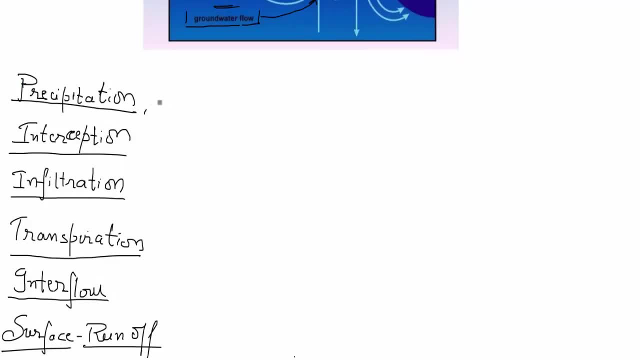 us look at what is precipitation Before precipitation. there is one more thing: evaporation. So evaporation is transfer of water molecule from liquid state to gaseous state. Very simple: from liquid to gaseous state, It is from oceans to sea. 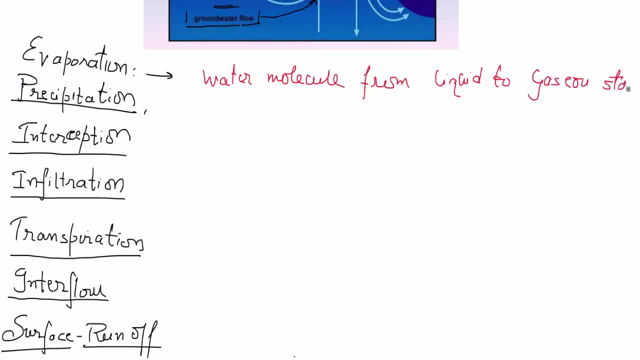 Now we have precipitation. This is deposition of water Deposition. it does not mean only rain. It contains all form of deposition of water on our surface from clouds. Deposition of water in the form of either rain or snow, or you can say hail or frost or anything like that. 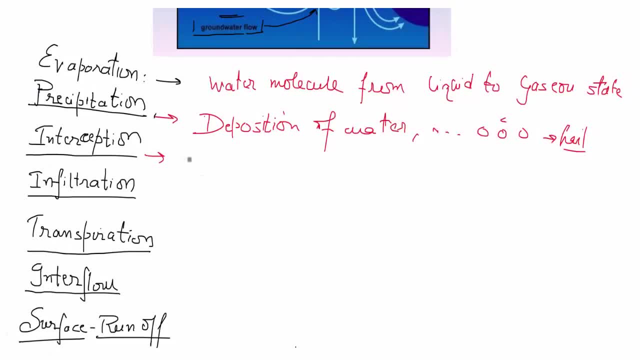 Now we have interception. Interception is suppose there is clouds and it is raining. So if there is tree, then over the tree and other vegetation there will be interception. Interception means water molecule will not be able to reach the ground surface. it will will be intercepted by this, this vegetation portion, this is our cloud. 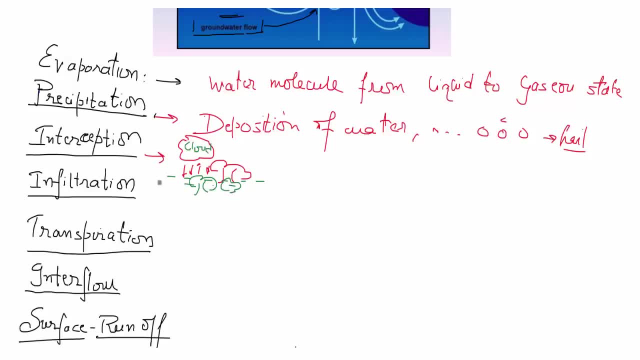 it is raining and it is our vegetation. it does not allow water to reach ground surface. now let us see what is infiltration. it is the movement of water through the earth surface in the earth. so basically this is our ground level. so if rainfall is coming here, then the water which which circulates down. 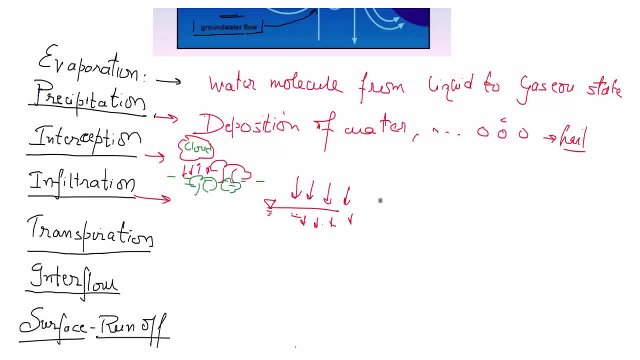 below the earth surface. this process is called infiltration. infiltration- transpiration is the soil moisture token up through the roots of plant and discharge into atmosphere through the foliage by evaporation. it means we have a plant system here. this is our, these are our trees. we then leaves and it has its 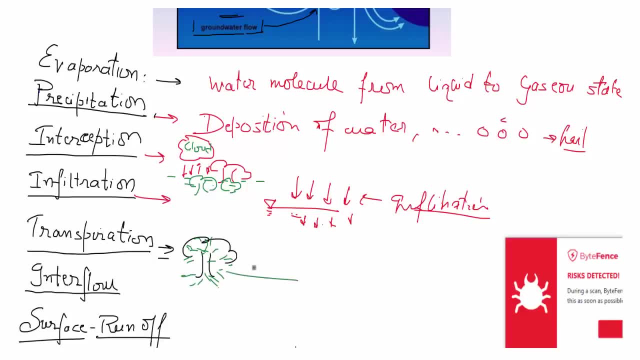 root, so below the ground level. so below the ground level its roots are taking water from the available motion and this water is going upwards the tree and through the leaves it leaves the earth surface. now you can say it evaporates. so this process is called transpiration and the 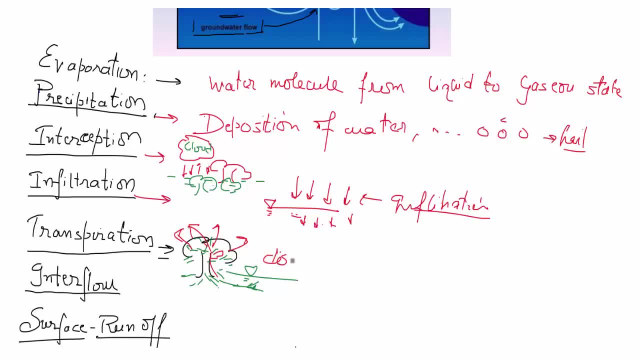 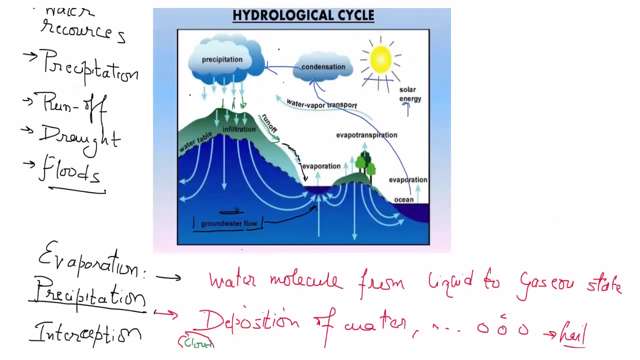 discharge of moisture into the earth, sir, into the atmosphere by the plants and trees, discharge of my soil moisture into earth's atmosphere, into the atmosphere. now we have inter flow. inter flow is that thing and like, suppose you have groundwater here and this groundwater if it meets, if the water comes through, if it's water there. 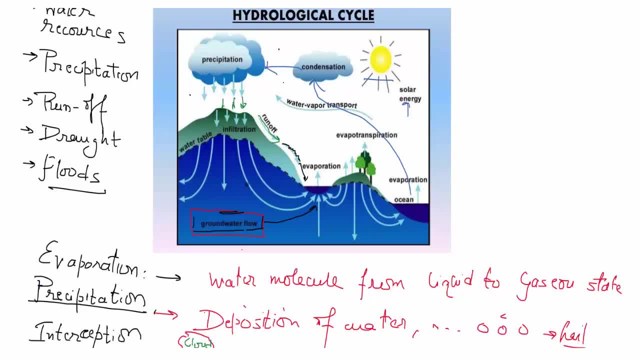 infiltration. it means water has infiltrated into our surface, but again this water goes on to meet. any other water body comes to the surface, so it does not. you can say these two paths: this path that is coming through the ground surface and this path coming over the ground surface. 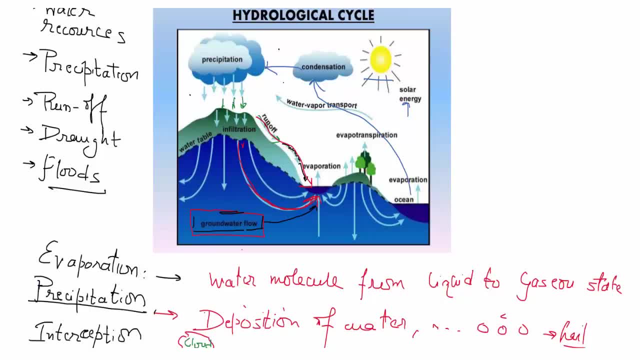 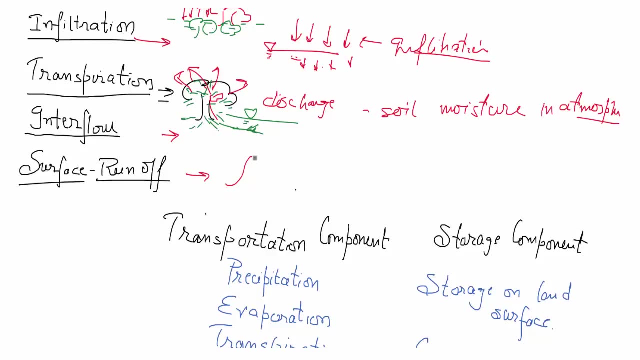 these two paths are: first, this is known as runoff and this is known as inter flow. this inter flow and surface runoff, as I've told you, there is a mountain and this is our river. if rain is falling, it will go a surface, or if there is percolation, it goes as inter flow. so 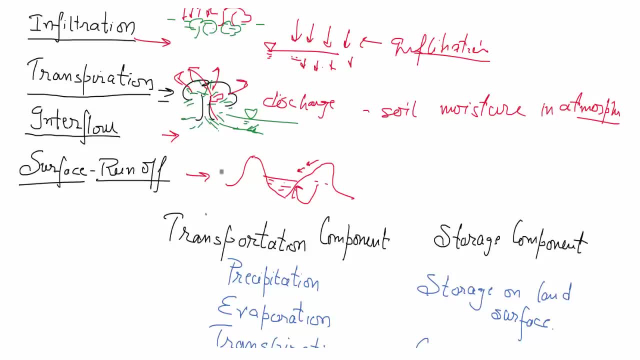 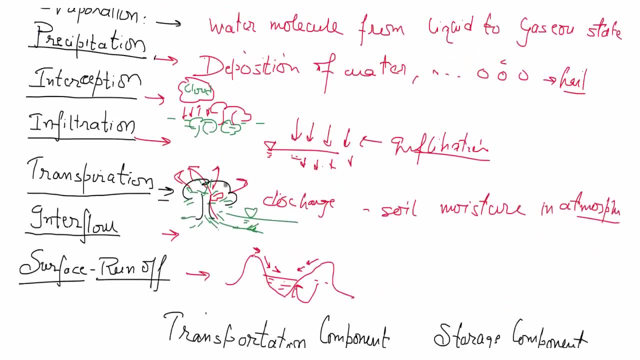 this is known as runoff and this is known as inter flow and this is known as surface runoff is that part of water which is drained at the outlet or of a catchment. this is known as outlet. this is our catchment area, which I will explain that. so we have seen basic hydrological process and these terms are: 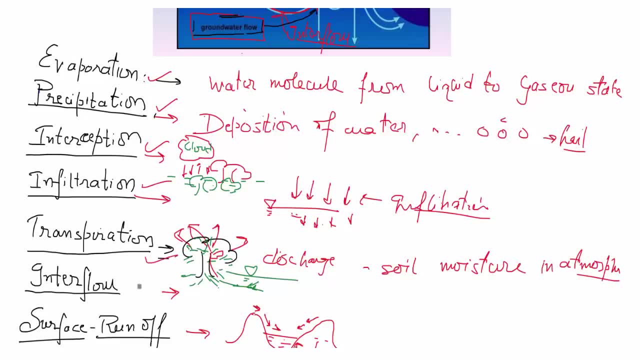 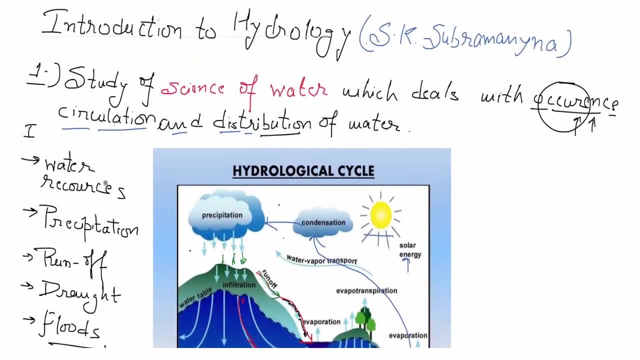 important for understanding the basis process because we will be using specifically, like infiltration and water flow, this is known as outlet, this is and surface runoff. these terms will be used frequent in analysis of our concepts. also, we will be looking at how the various water sources managed through. 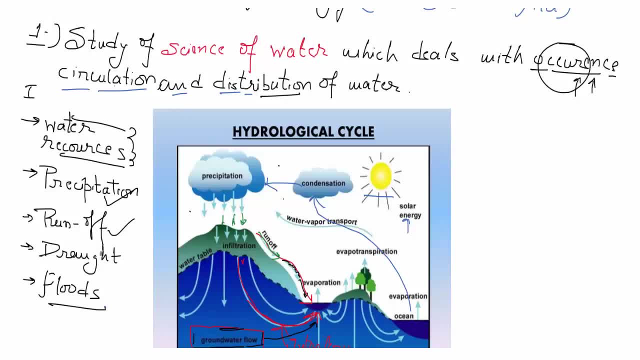 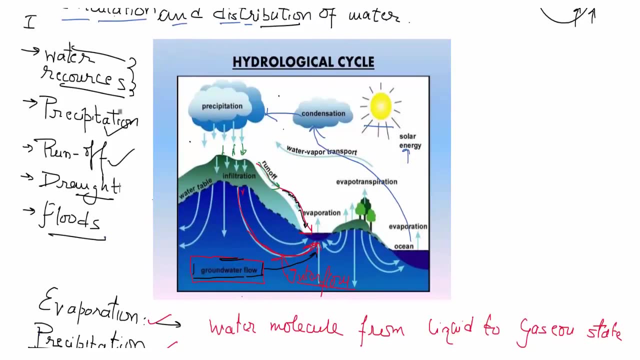 the study of hydrology, how we can calculate precipitation, runoff and how we can predict drought or floods in case of, and we will also be looking at some models to predict what will be like kind of situation when there is when, when there will be flood or what, what situations can lead to drought or how. 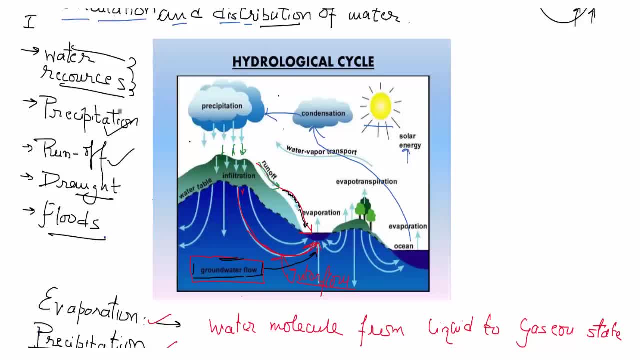 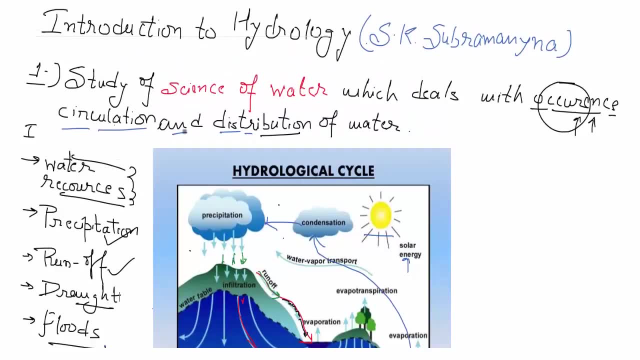 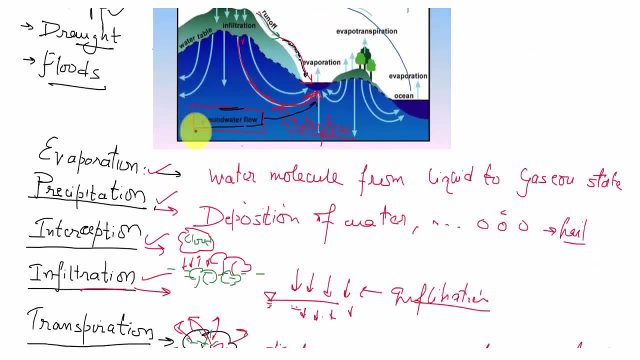 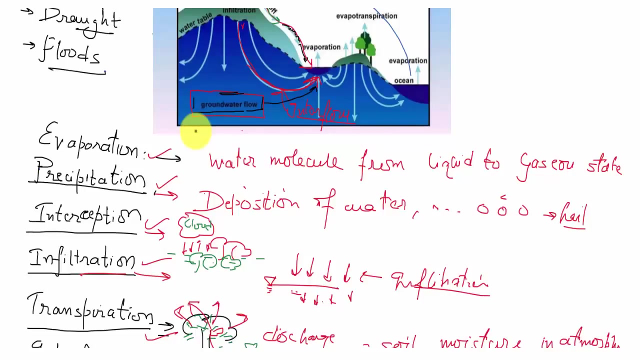 much water is essential for farming and these things like that. so in this lecture and in the series you will be getting basic idea about this concept of hydrology and this can be used for your study in courses of civil engineering, such as your classroom study. your kind of question for examination- it will cover. 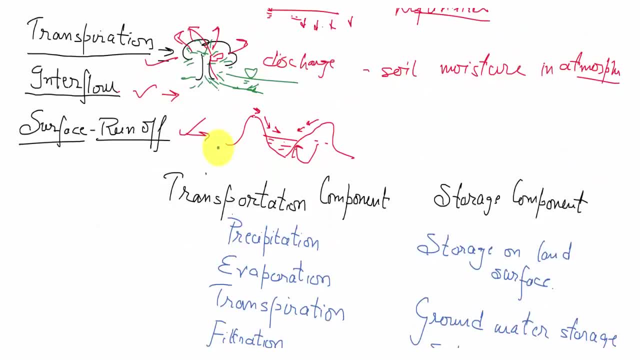 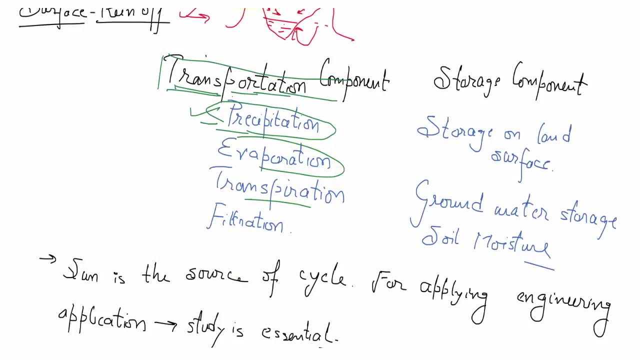 almost every aspect which is related. so now let us see transportation component and storage component. transportation component mean how the body, how the water, can move. so we can see water moves through the fresh, precipitation, evaporation, transpiration, filtration. this is, these are the various ways through which water 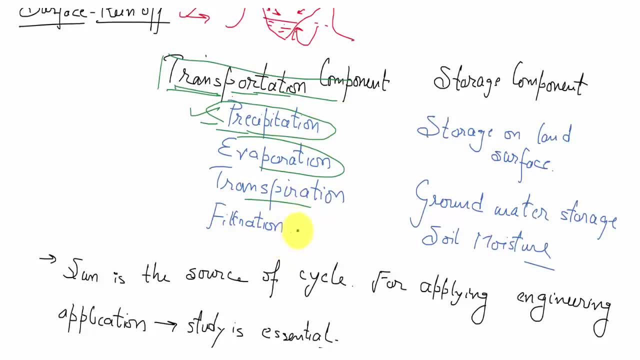 molecule or the one form of water moves through one place to another place. now, storage component means: what are the various ways in which water can be stored. so water is stored on land surface means either in pond Lake, River or ocean. these are the water flow phase, and so water flows in different ways. so we winter water and we water from other places. 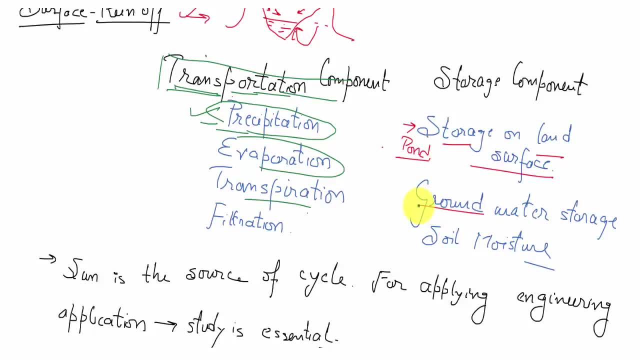 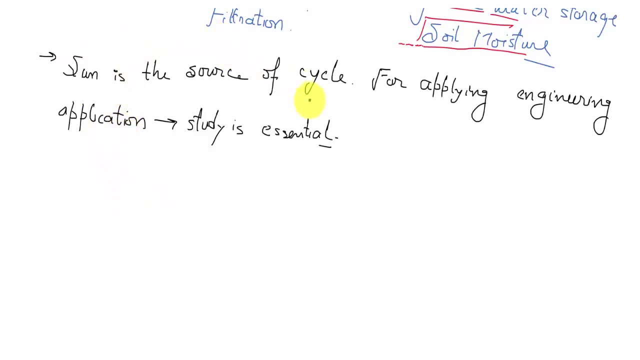 storage component on surface, it also gets stored in groundwater and, last but not least, as water is also stored as soil moisture, as we have discussed earlier that all the hydrological process only occur in the presence of Sun, so our energy is derived from Sun and there is no gain or loss of 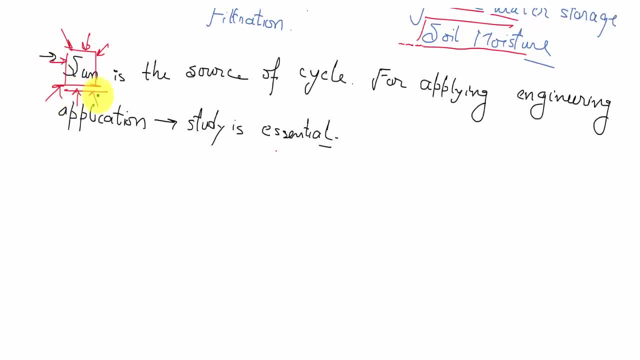 energy. only one energy is converted to another form. so, keeping this in mind and other aspects for applying engineering applications, we can say that study of hydrology is absolutely necessary for managing water resources and understanding the basic cycle of water. now let us come to a very interesting 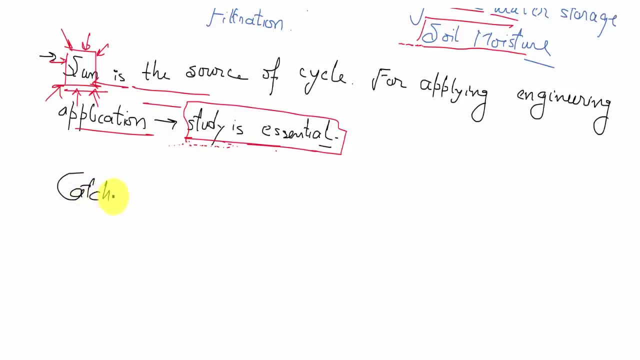 concept which is called as catchment area. catchment area, as you can see, by name, only we have that. it catches something. it catches what it catches. it catches water or rainfall, or precipitation. water or precipitation, basically, it is in used in concept of rainfall or stormwater. 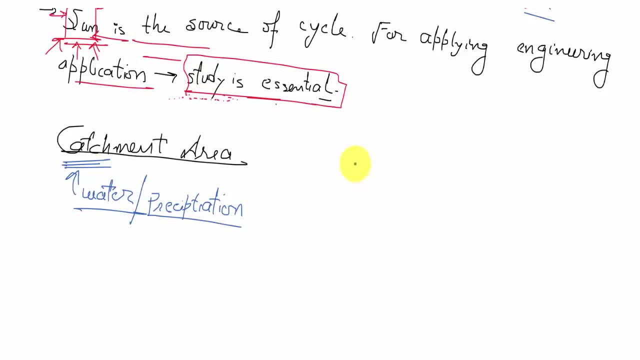 let me say that this is our mountain. I am showing you elevation. this is also series of mountain and you can say these are- this is your kind of a valley like thing- very steep mountains. so if what will happen, and you know there is a river going through this mountain, at the base of this mountain, which generally 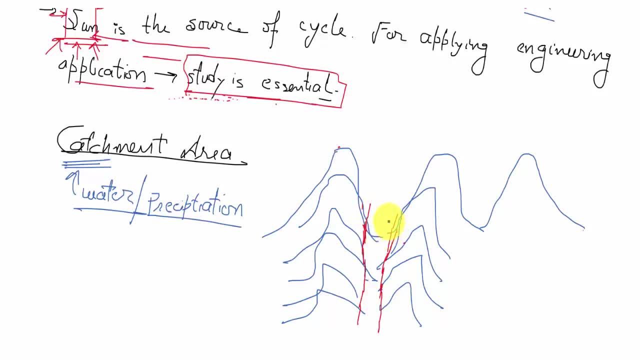 the case in most of the most of the water system, there is a river which comes down the slope. now, if rainfall takes place, then we will see that all the waterfall which comes which falls on this area, this it will drain here, it will drain in this river. only I am just trying to give you an idea what called rainfalls which bigger there. when rain falls critically places there, you will problems. now we will see that all the waters which falls in This area is�m experiment with waterWater mouth. 먼저 nuo cape tarp run znajup anão na Patience este. 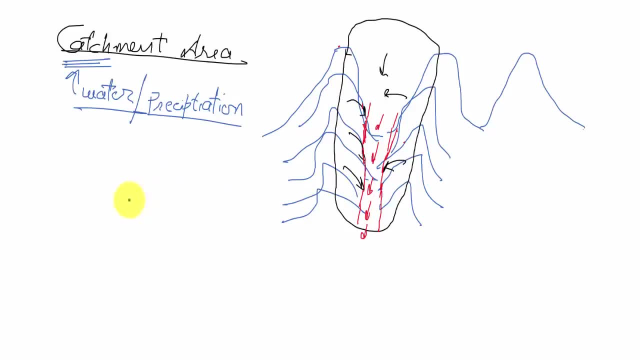 idea that what does a catchment area mean? well, let us start with a simple concept: catchment is that area. catchment is basically an area which drains into which. in drains. into drains means all the water falling in this area will come. here means whatever the river it is flowing and or any any source of stream. 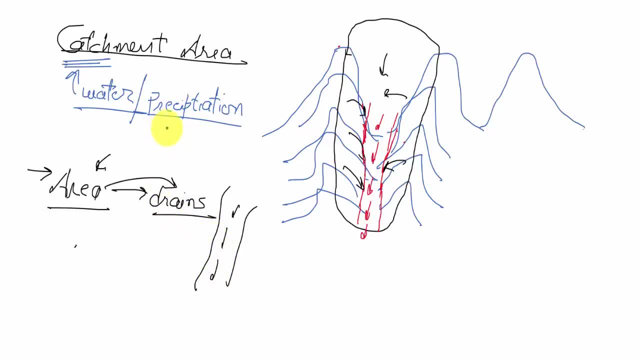 so if this, if all this area, drains into this river, if all the water falling on this land will come in this river, then we can say that this is our catchment area, this, this, will your catchment area. let us you can say that there are few more terms to denote catchment area, such as drainage. 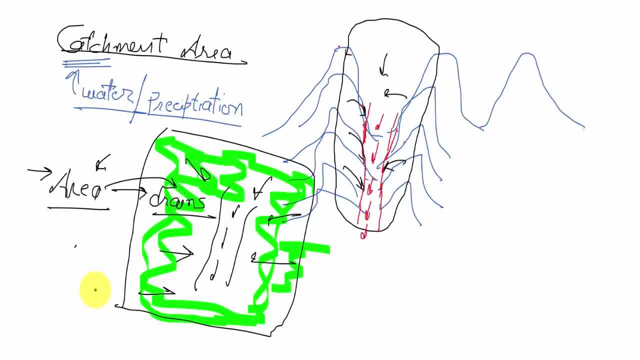 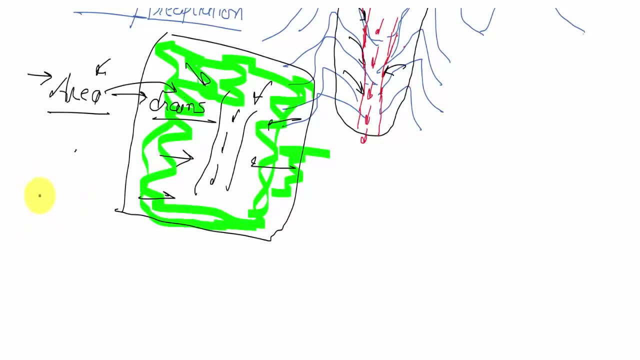 patient, catchment, basin, drainage area, river basin, water patient- all this thing basically mean the same: that water over the area is where in Paul is falling on that land, it will drain into a particular river or a stream of water. now we look at what is called as water shed, divided. 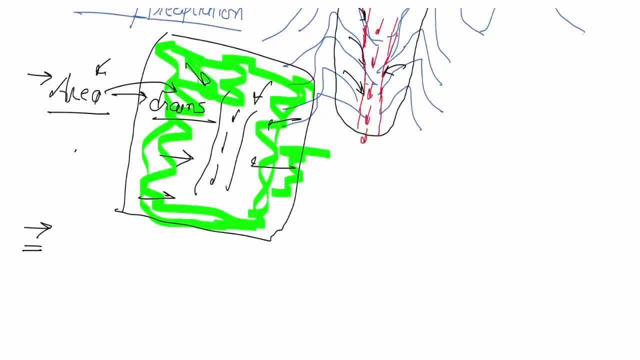 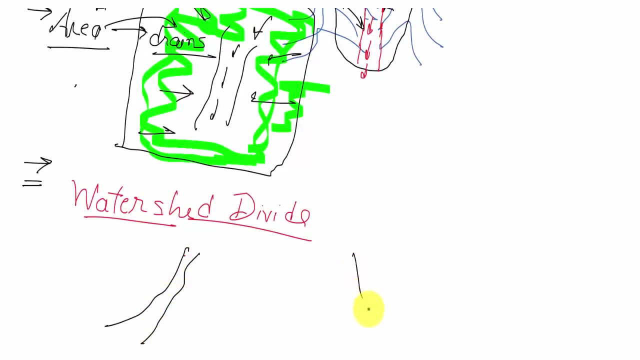 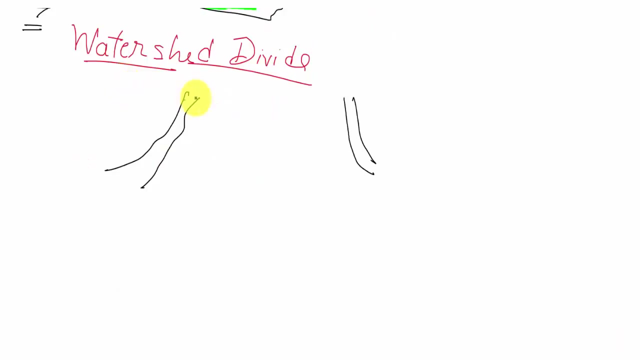 or topographic water divide. watershed divide is that concept which says that which separates two catchment areas. let me tell you basically, suppose we have one, we have two rivers flowing like this and another they were flowing like this. so if, if we have this is our watershed divide, this line. so if rainfall, 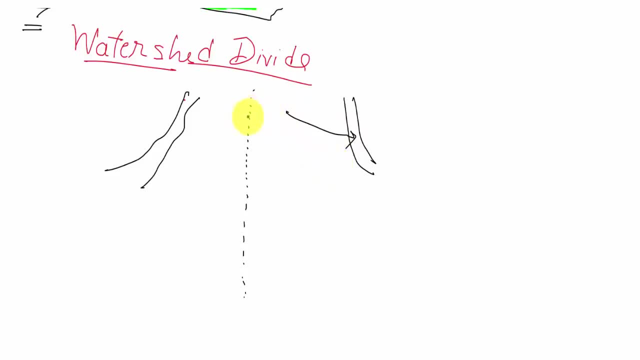 falls, here it will meet. go and meet this river. if rainfall comes, here it will go and meet this river. so this line will become what is called as watershed divide. it will divide two catchment areas. basically, this divide falls generally a ridge line means it is a meeting point of two mountains. here is 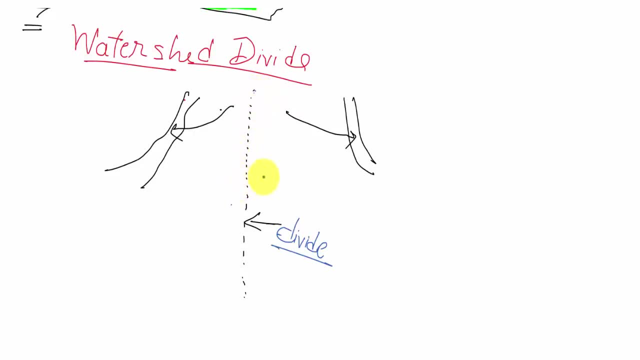 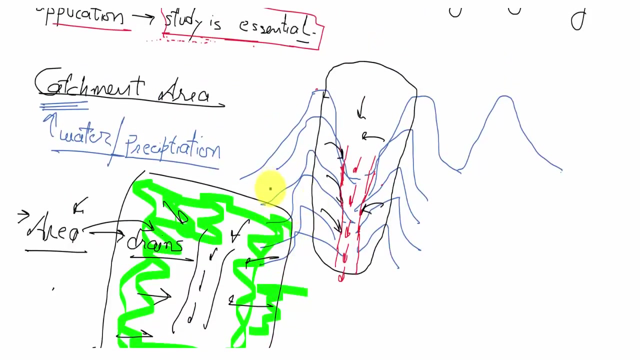 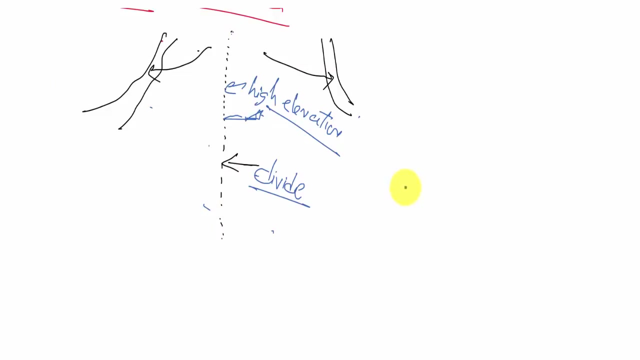 or it is a ridge. it is a high, high elevation area, high elevation. it has high elevation as compared to both both of these river. now I think we have understood what is catchment area and what is watershed divide. so let us move ahead and let us look at what is called a catchment leakage. catchment leakage is: 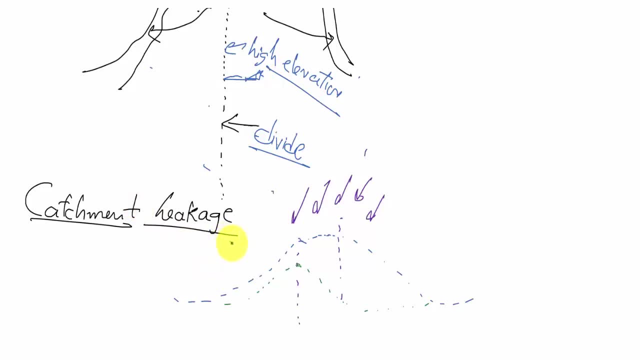 a concept which explains that if this is our- let us say it is our- watershed divide, this, this, this divide is called as what freshman device? so if rainfall falls here, half the water will go here and comes here. it will come here, but if this is a called as our groundwater divide, 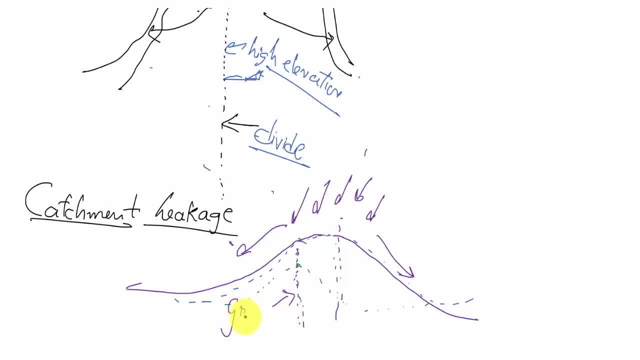 groundwater divide. it means it separates the flow of groundwater with respect to put the streams down, water divide. now, if water comes in this portion, because there is difference between this watershed to pour up with, water divide and groundwater divide do not match in some cases. so if water comes here, fall. 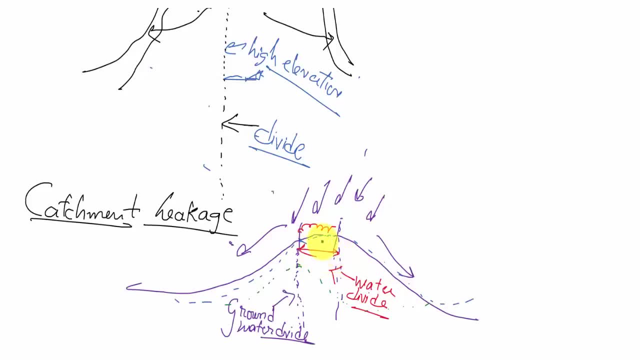 in between these two. you hide, then it is most. then what will happen at water will come and meet here, water flow will occur like this, water flow will occur like this and we meet a stream somewhere here. so what has happened? that what it was part of this watershed divide has. 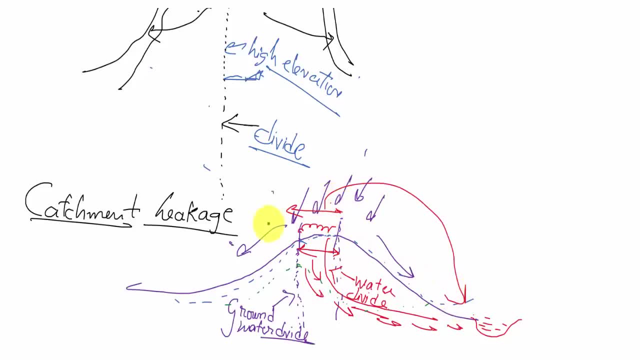 come to this, so this is called as catchment leakage means this water has leaked from this water amount has leaked from this side of the catchment area, which happens when groundwater divide and topographic water divide does not match for large catchment areas. this leakage is neglected and these two lines, these 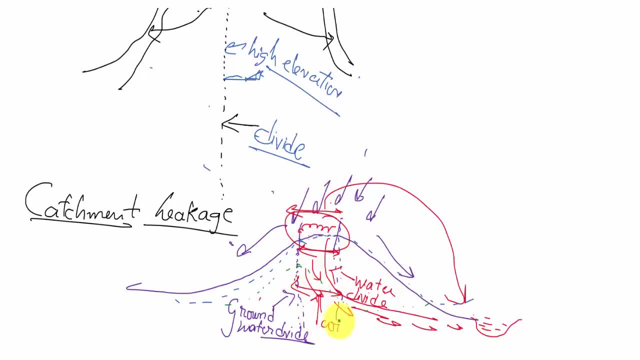 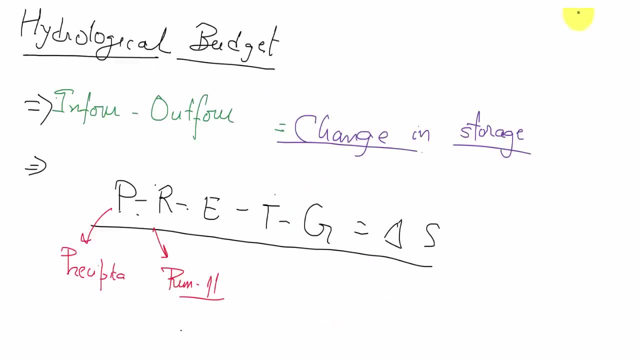 two lines to coincide. hydrological budget equation is basically continuity equation. is also called as a water of budget equation. it says that whatever water is coming means whatever is coming, it is coming. this one is the water that is coming means that whatever is coming means whatever is coming, this one is coming. 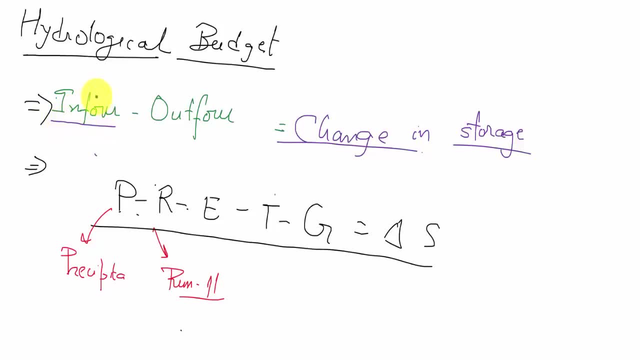 means whatever water is coming in dam or river or any water body is called as inflow and whatever water amount is going out is called as outflow. so water which has come minus water which has gone out will be equal to change in storage. but if 7 meter cube comes and same amount of water goes, 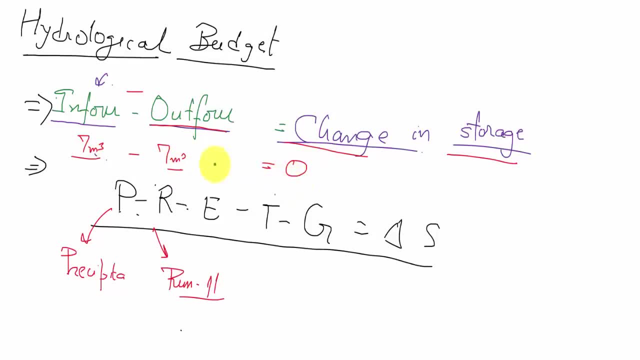 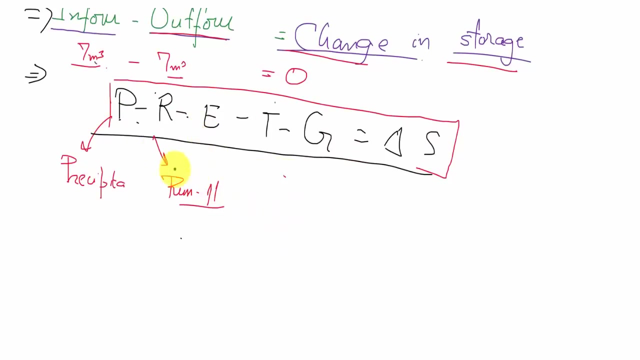 then there will be no change in storage because there has not been any addition or subtraction of water from this water body. we can see this equation in detail. this is a detailed water budget equation. this is P. P means precipitation. precipitation is whatever the water is being added. 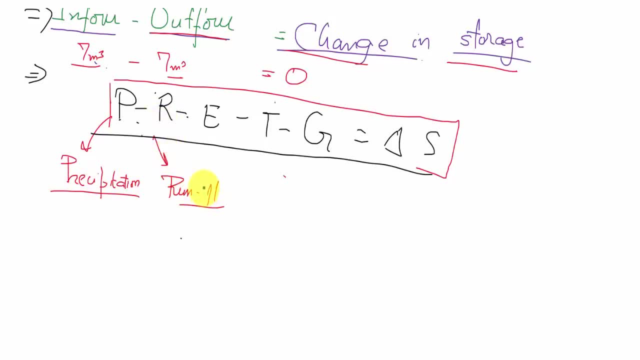 now R is runoff. runoff means whatever water has been lost. E is net evaporation. whatever water lost due to evaporation: T is net transpiration. transpiration. water lost through leaves of the trees: T is net transpiration. water loss through leaves of the trees: T is net transpiration. 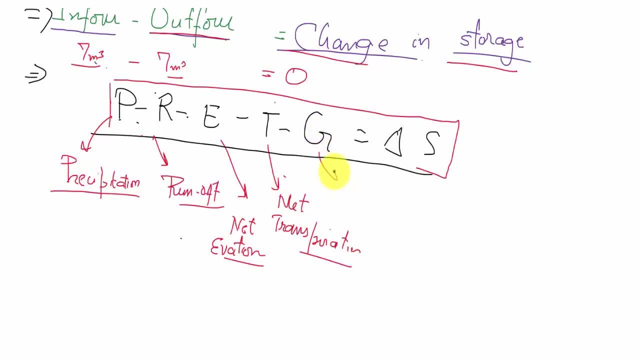 T is betfiguration, T is betfiguration. T is better than fish, t is better than�� think. it means it had not been that much water because we are on would be a Kirchberg cocktail. we are our grandson now. inflow minus outflow. you can label this. this will be our inflow and this. 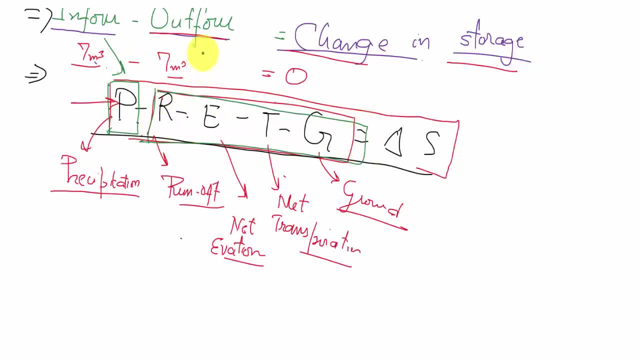 term. here is our outflow. outflow consist of a runoff, evaporation, transpiration, groundwater storage and this net will be equal to change in storage. either it will increase or it will decrease. depends on which term is greater or lesser in terms of rainfall equation: rainfall runoff equation. that is a very 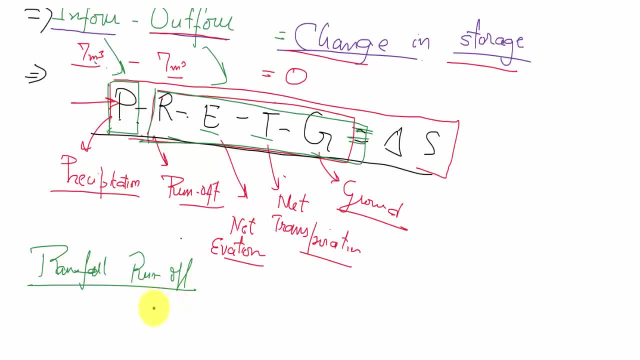 simple. we say that there is precipitation minus loss. whatever losses are there, it will come in it or is runoff, whatever water has run away. so okay, so let's see what is the precipitation and the loss in the water. okay, so let's see what is the precipitation and the loss in the water. 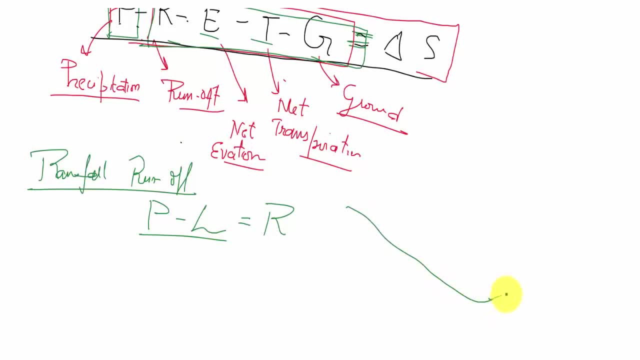 whatever water is falling here and whatever water is lost. finally, the thing which reaches here is called as runoff and the total amount- q suppose q amount of water has fallen and it will be q dash, because these two water is not same. it is loss in the form of, as i told you. 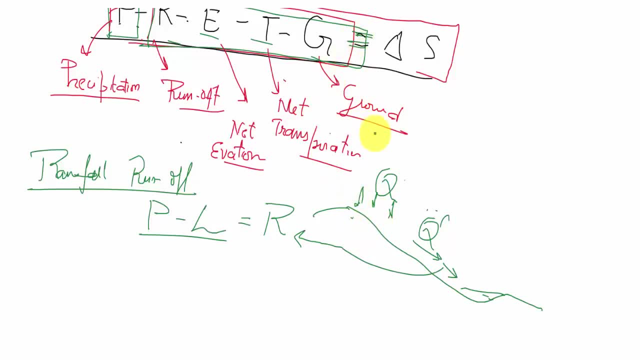 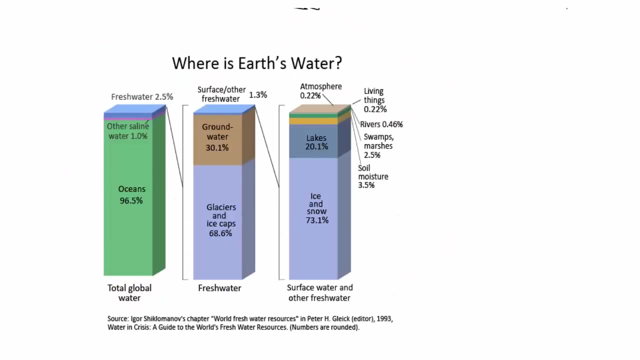 transpiration, infiltration, percolation, groundwater, sewage change. so this is our rainfall runoff equation. it is an important equation. we will be using it later classes once again. let me write it like this is: runoff is equal to precipitation minus losses. runoff is equal to precipitation minus losses. now let us look at the global water balance. 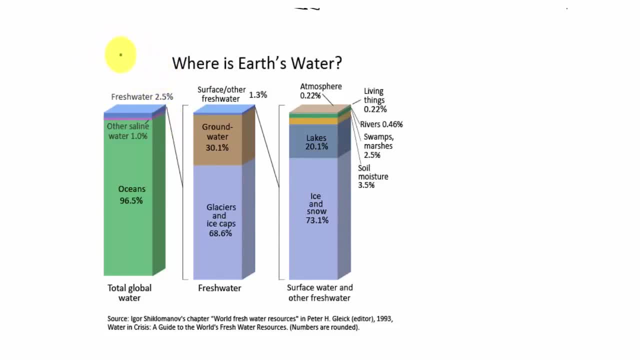 global water balance basically comes to a point where we have to look at what is the distribution of global means, earth's water, in what form these are stored and what are the various percentage according to which they occur. so, as we know that most of the water on earth is in oceans- 96.5 percent- and it is a saline, very big saline source of water. basically, 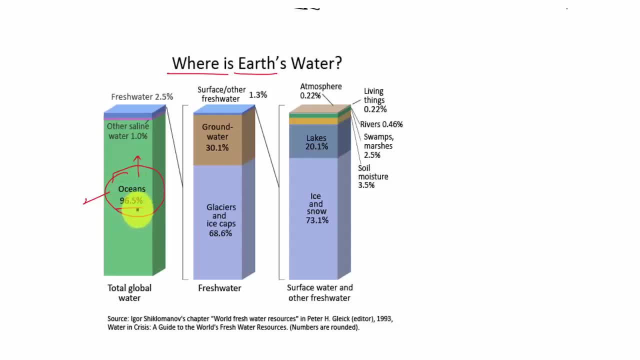 we cannot drink ocean water because of high amount of salinity in it, and this does cause a major global water crisis problem- that we have so much water but we cannot use this water as a drinking purpose. so our 96.5 percent of level water is in oceans. 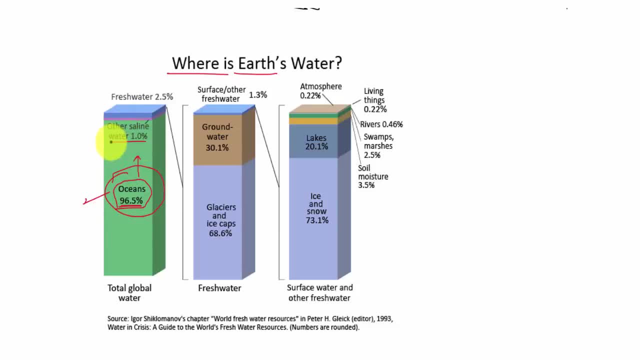 and it is a saline. then we have other saline sources of water which constitute about one percent, such as lakes and other saline water bodies. then we have a fresh water, which is only 2.5 percent of the available water and water on the earth's surface. now let us see distribution of 2.5 percent. 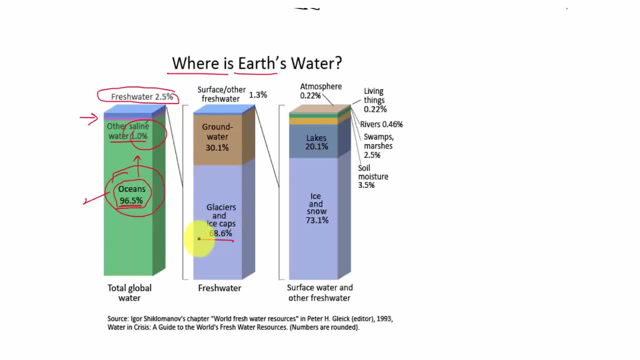 fresh water. out of this we have glacier and ice caps. we know that we have two major ice caps- north and south pole- and surrounding areas. so we have big concentration of glaciers and ice caps on both the surface of earth surface, on the north and south pole, which constitute around 68.6 percent of fresh water. 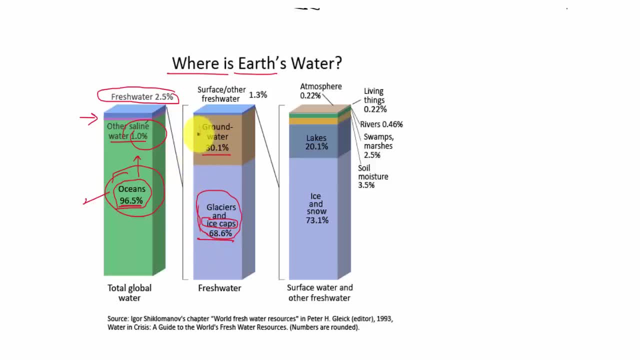 then we have 30.1 percent, which is fresh water stored in ground water, and now we have 1.3 percent of available fresh water which is stored as surface water, other fresh water. now we can have a look at distribution of this 1.3 percent of fresh water out of this ice and snow. 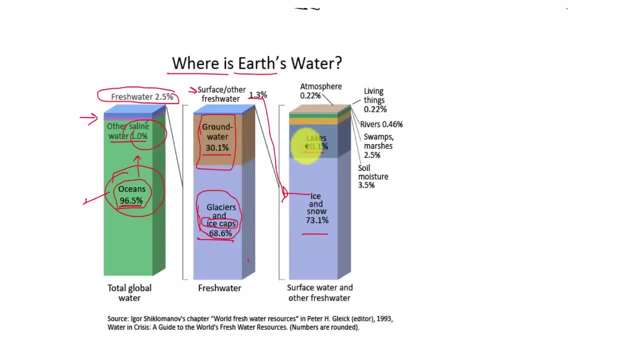 constitute 73.1, lakes constitute 20.1 percent. now we have swell, moisture, river swamps, the living beings, atmosphere, all these thing in very tiny fraction, very tiny fraction, or a very tiny fraction, you can say, and we are passing through great changes. so at this point, because of the special structure and our most of consumption. so, basically, if we are 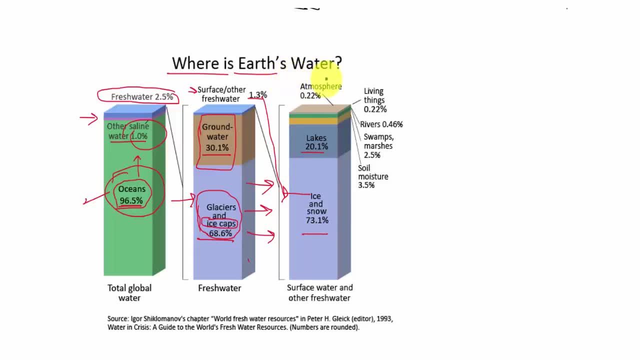 not able to generate adequate amount of fresh water for drinking and other purposes, then we will be looking at very bleak scenario where we are basic drinking water will not be accessible to most of the populations. Therefore, we have to look at the sustainable ways where we can either use- we can use those- 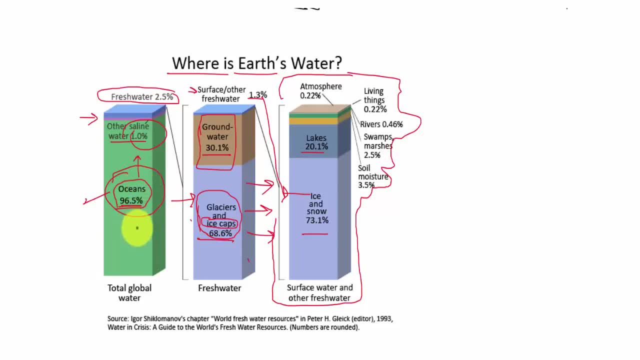 processes which consume less energy for cleaning ocean water, or we can, we can look at the ways of filtration and and cleaning our rivers and basically putting an end to polluting and and, most of all, we should. we should not waste water where it is not required, or even 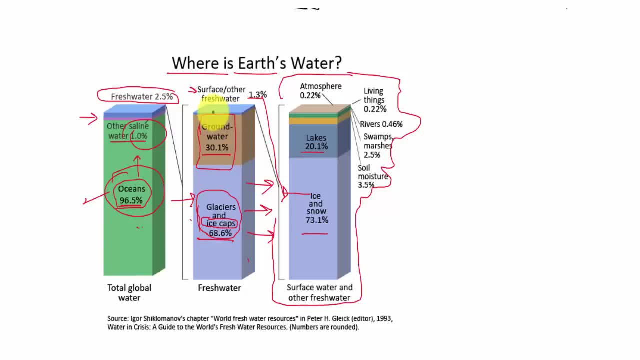 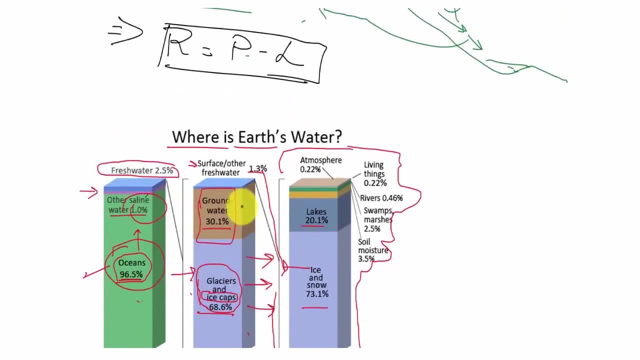 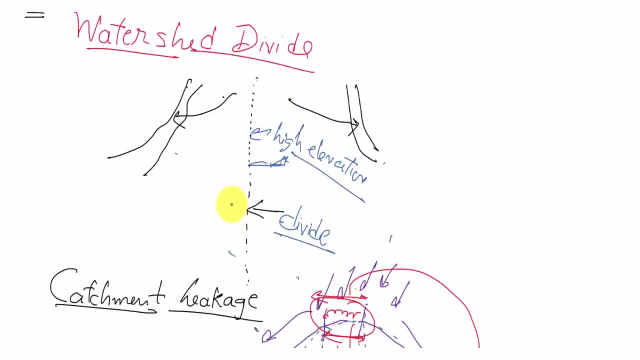 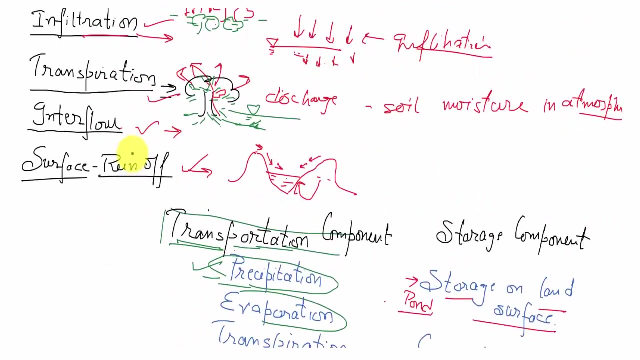 we should take care that all the water and all forms of water used by human should be in a very judicious manner. So in this series we have seen introduction to hydrological processes, where basically we have looked at hydrological cycle, Then at various terms, preparation, transpiration, like this. then we have 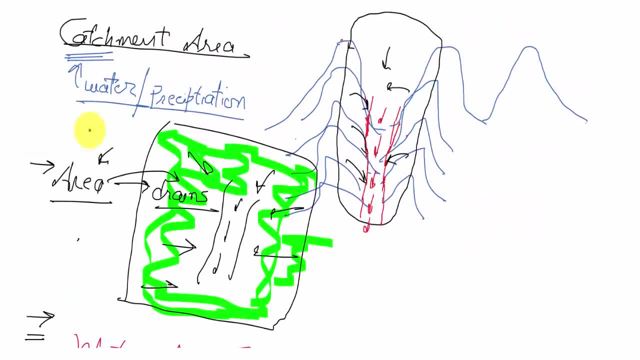 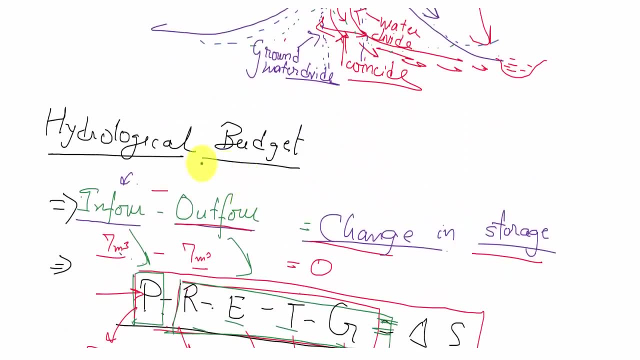 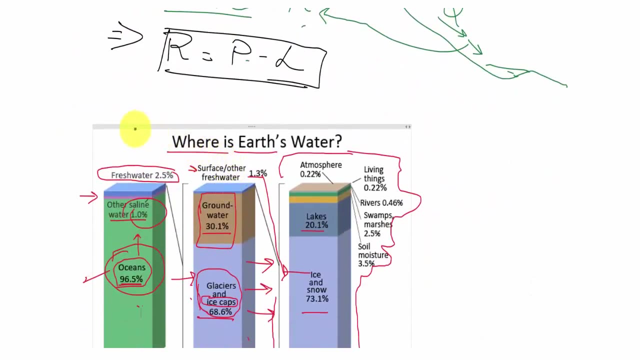 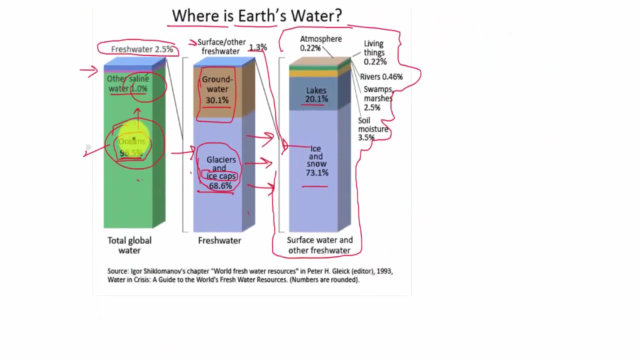 looked at catchment area definition and train catchment area divide what I should divide. then we have looked at catchment leakage and hydrological project equation. where is influence for chain storage? then we have seen arts water restoration. so let me know if is any improvement you would like to see or any. 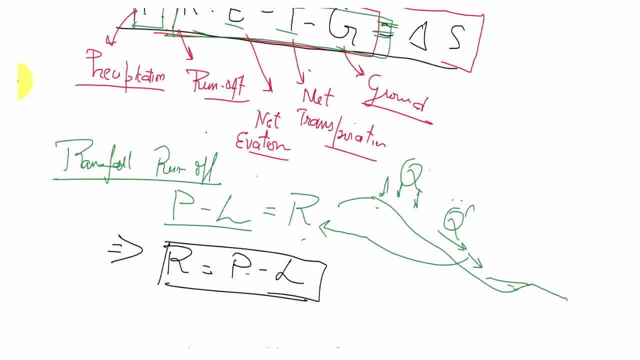 mistakes that I may have made, leave in comment section below. thank you.